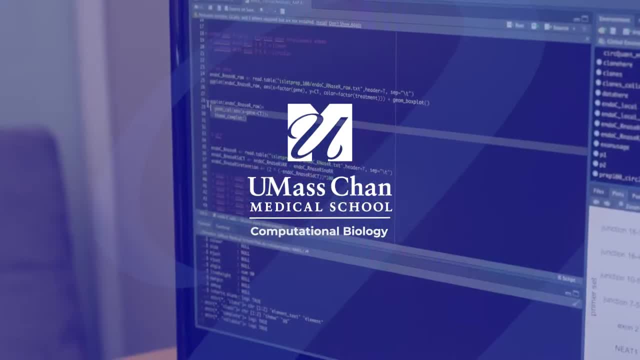 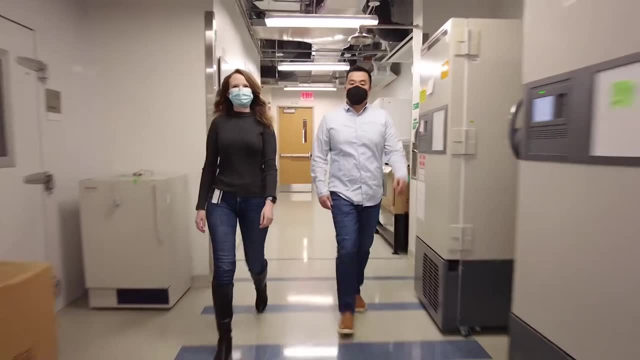 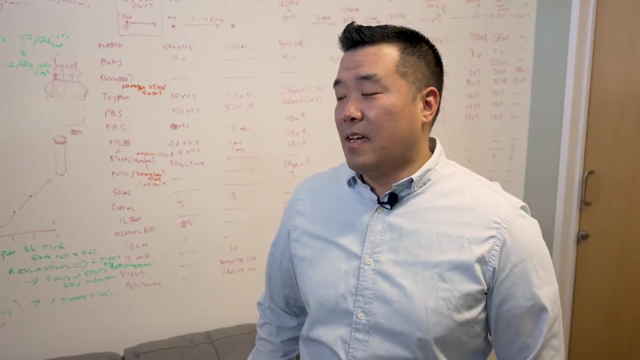 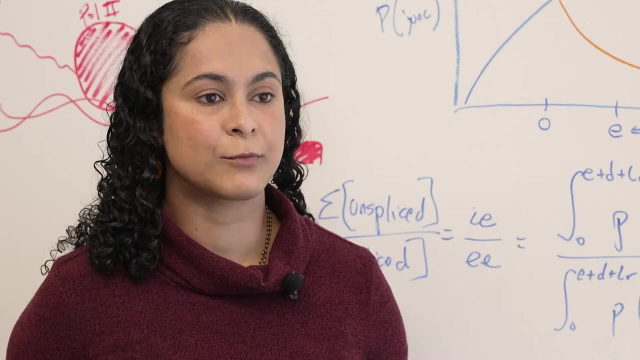 Computational biology represents a number of different related disciplines within the field of biology. What they share in common is their need for quantitative insights. This includes things like genomics, bioinformatics, statistical modeling or mathematical modeling, all of which are becoming more heavily represented in the field of biology today. My lab studies the processing of 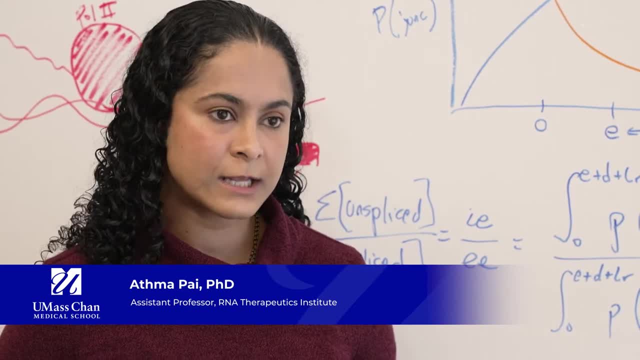 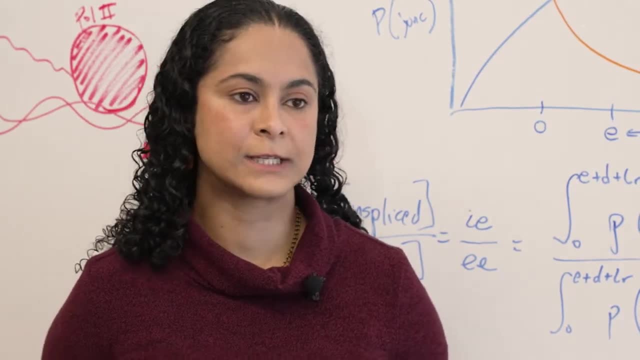 mRNA, essentially how mRNA gets created, can get processed and ultimately becomes a functional molecule. And to do that we use both functional genomics, very high throughput techniques and a fair amount of computational, statistical and mathematical tools to analyze the data that 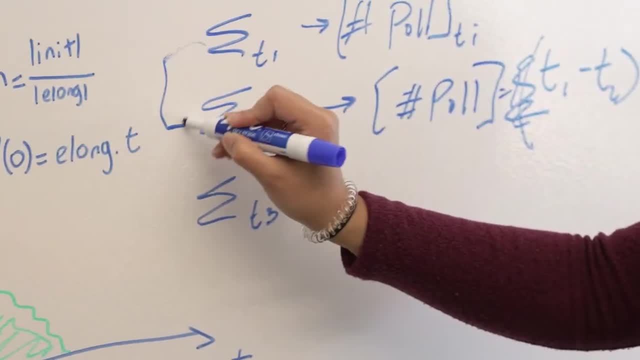 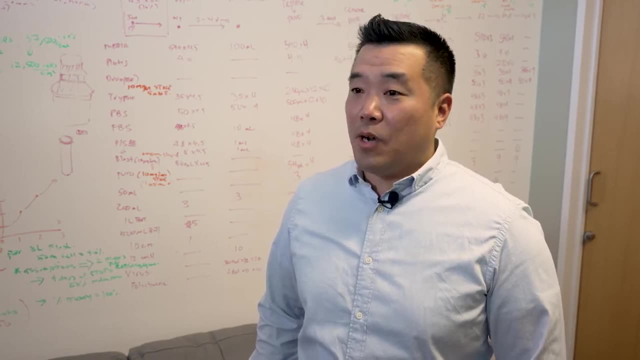 we generate, I think over the last 20 years, what we've seen is that the nature of biological data itself is really quite. it's really changed quite a bit, going from things that were really quite qualitative in nature- us describing or observing things- to us really wanting to put discrete 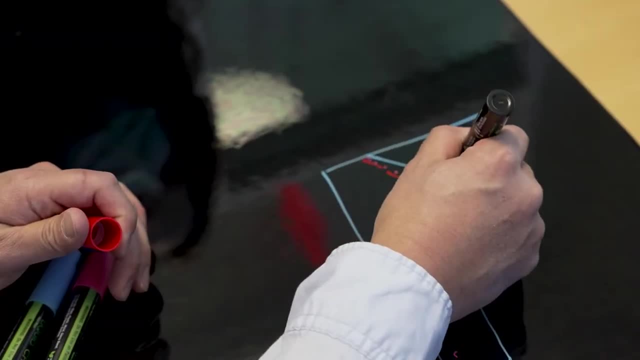 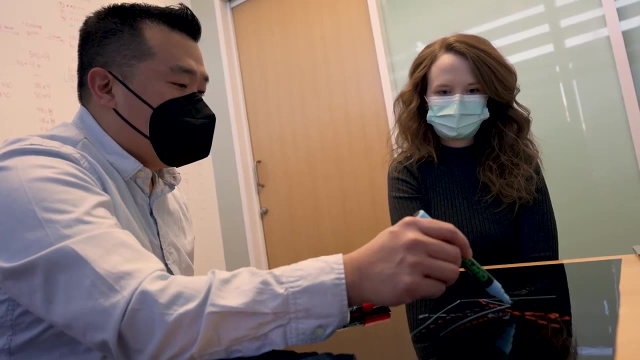 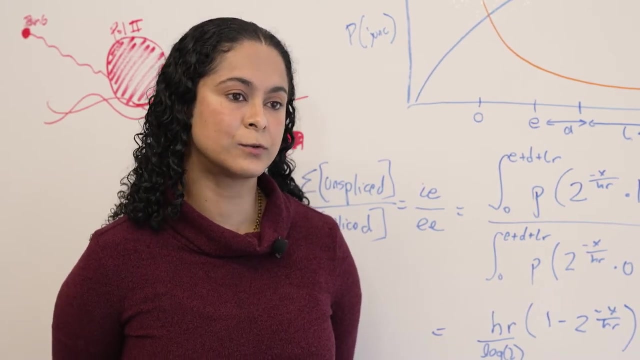 numbers on the things we're seeing And then, by looking at those numbers, seeing that there's opportunities to be had, opportunities to learn more about the underlying processes that drive biology. through the quantitative insights, There is an understanding and an increasing appreciation that using both quantitative and computational tools to actually analyze the data will allow. 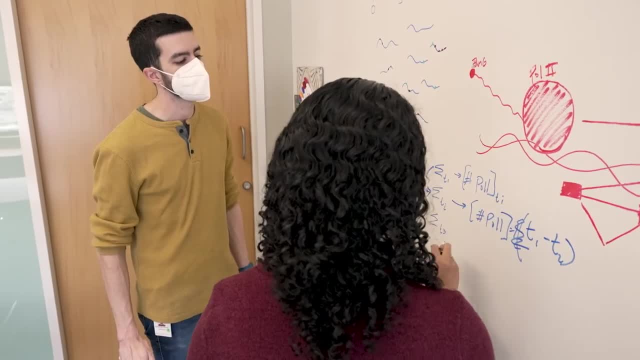 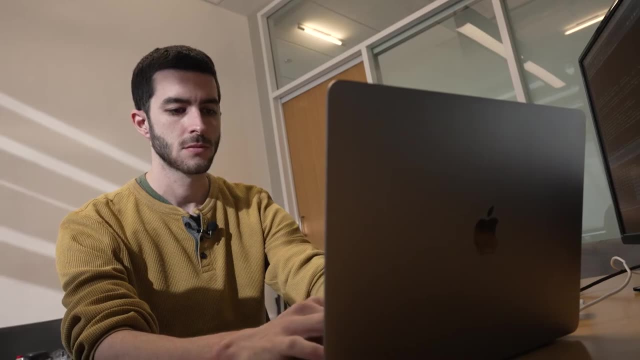 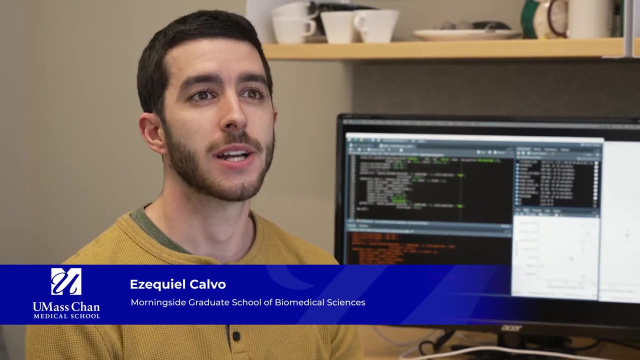 you to both test hypotheses but also generate many new hypotheses, And that's why I think it's becoming an increasingly appreciated tool on campus. When I finished my undergrad, I knew I wanted to do computational biology, but most of the programs required some type of experience and I didn't have anything. So UMass has this umbrella program. 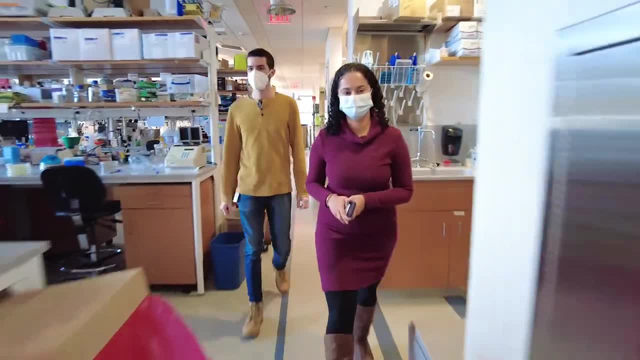 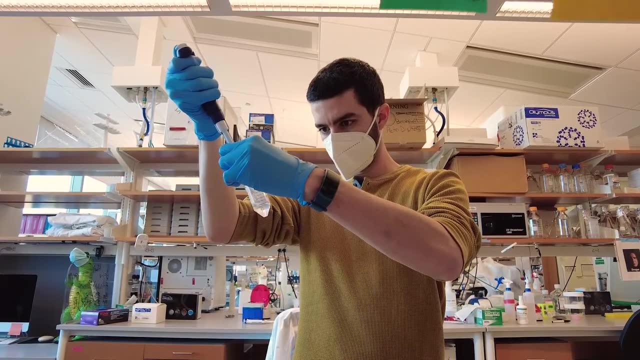 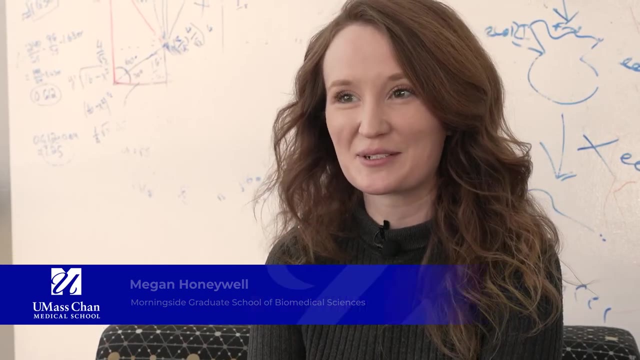 that allows students from different backgrounds to do computational biology or any type of science at all, So that was a good start for me. I was a biochemistry major in undergrad, so it wasn't really something that I considered as a possibility in undergrad, But coming into grad school, 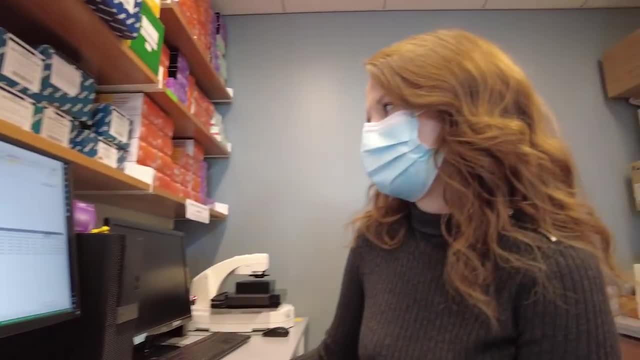 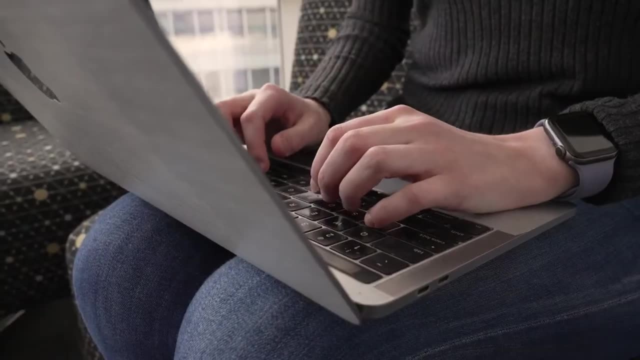 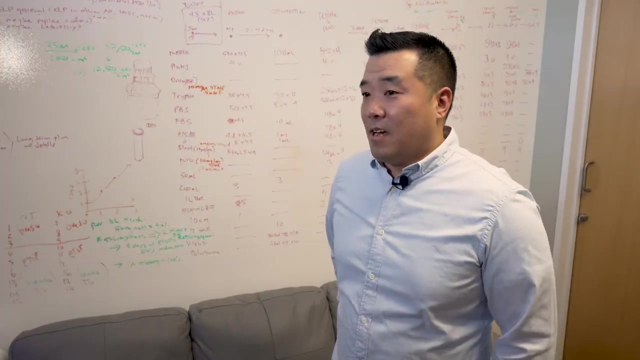 UMass, I think, has a really great infrastructure for taking people from no experience to having a lot of experience and considering themselves computational biologists. If we give basic training to people with good biological intuition and good biological training, what we're often able to see is that the students can unlock a really unknown competency. 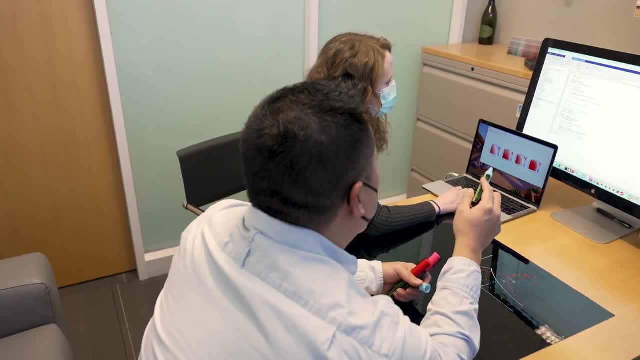 that they're really quite talented in these areas. Most of the students in my lab came in with a lot of experience in computational biology and they were able to do a lot of things. Most of the students in my lab came in with a lot of experience in computational biology. 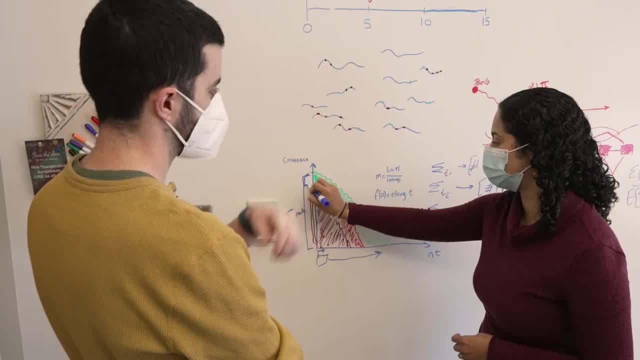 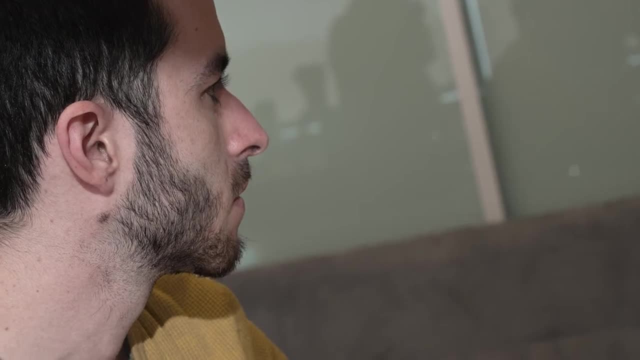 Most of the students in my lab came in with very little programming or very little computational experience, but are certainly getting a ton of experience on the ground, And I think that's in some ways the most practical and most fulfilling way to actually learn some of these skill sets. 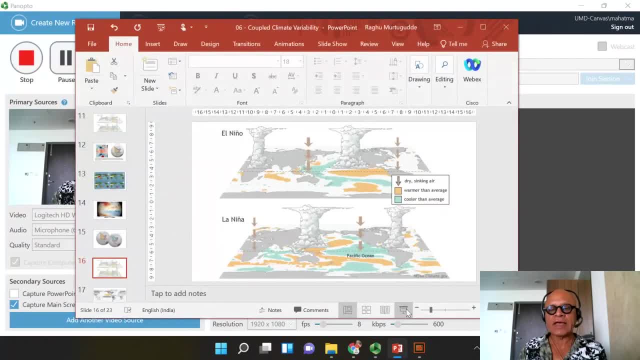 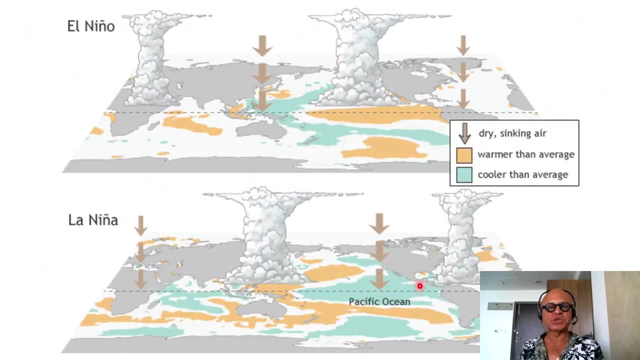 So let's conclude this chapter with what happens in the other oceans. So we always look at El Nino as the poster child for explaining ocean-atmosphere interactions, mode of climate variability, how climate variability affects global teleconnections, and so on. 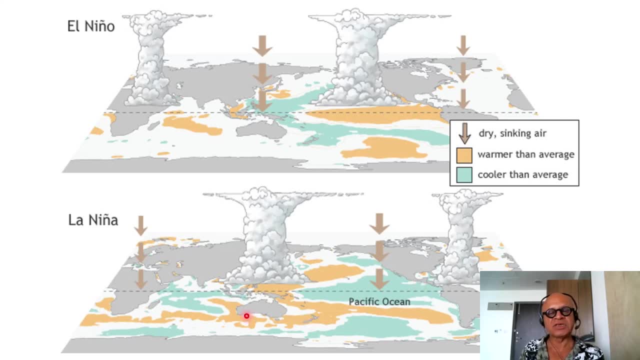 So if you look at this map, you see the curious changes in the tropical circulation as well, right During normal times. you have deep convection here and you have sinking over here. This is the Pacific Walker Cell. You have sinking over Western India, Eastern Africa, Western Indian Ocean, Eastern Africa, which is the Indian side of the Walker Cell. 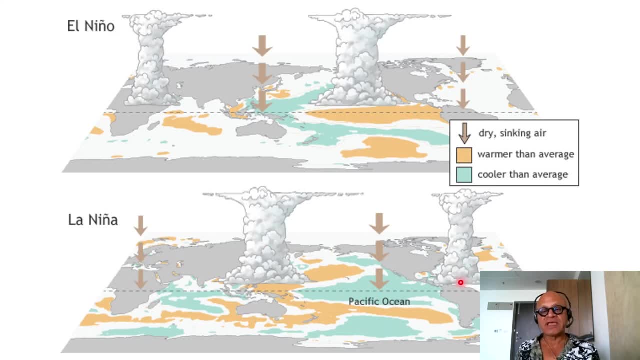 And of course, you have another convection center over the Amazon, And West Africa has a desert, West Africa has a monsoon as well, So but the main thing you would notice is that the zonal extent of the tropical Pacific is far, far, far greater than the zonal extent of the Indian and Atlantic oceans. 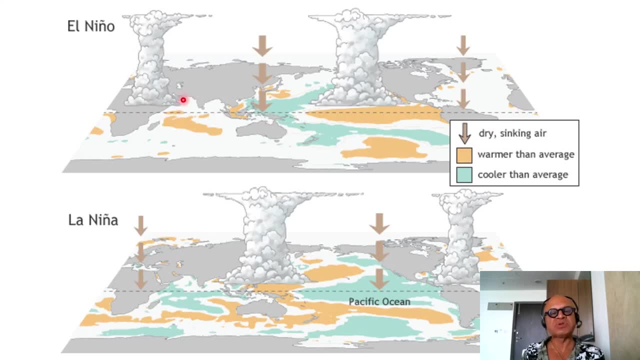 And we've talked about how the mean sea surface temperatures and rainfall distributions are dramatically different over the Indian Ocean because of the monsoonal circulation, which is North-easterly during the winter months, South-westerly during the summer months and inter-monsoons are rather weak, and so on. 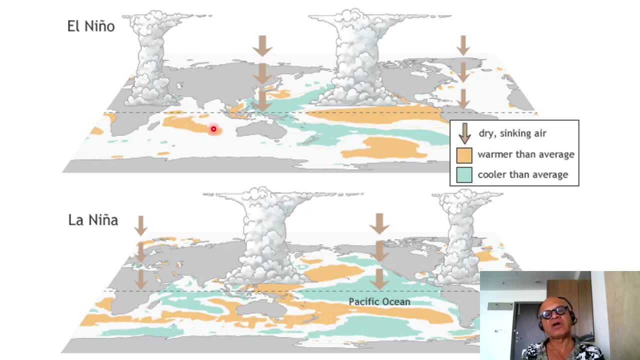 And the trade winds are mostly confined to the south of 10 south and so on, And there is no strong upwelling here. This is in climatological condition. the Indo-Pacific warm pool and colder temperatures happen here, especially during the winter. summer, boreal summer.